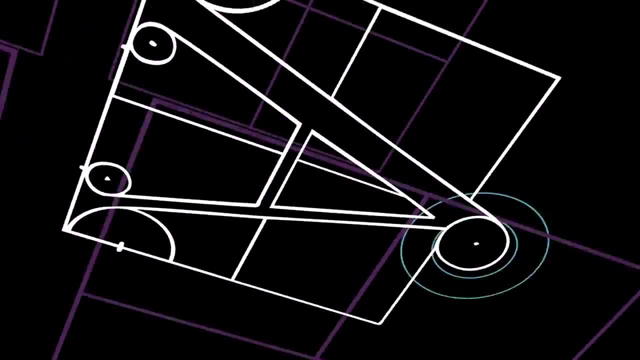 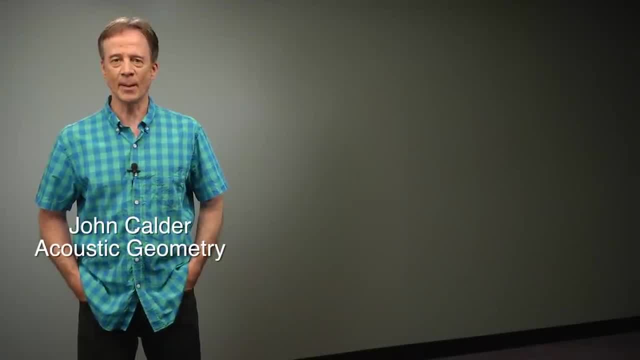 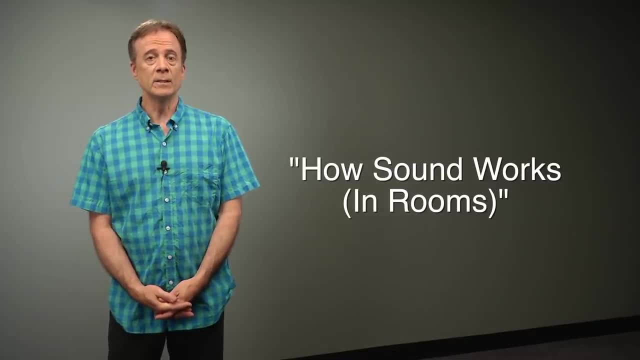 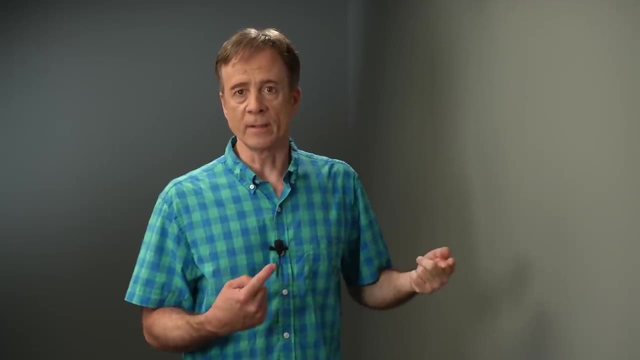 Hi, I'm John Calder of Acoustic Geometry. Let's talk about acoustics, which is basically how sound works in rooms. It may seem complicated, so let's make it simpler. Most rooms have flat walls and flat ceilings, and sound bounces off of these, So how does that affect the 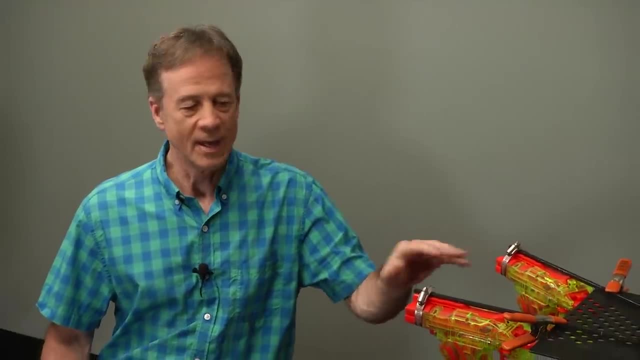 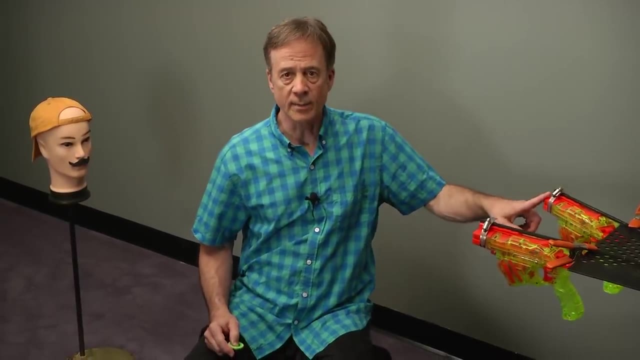 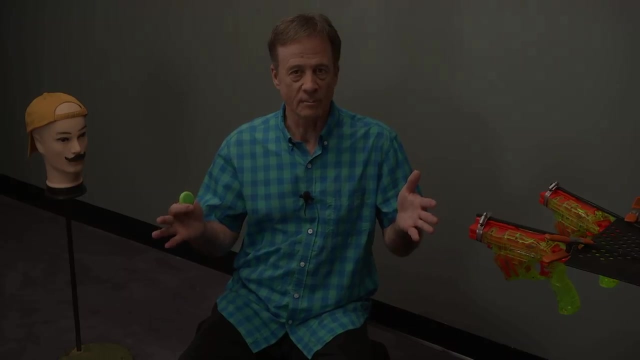 sound. I'll use these two Nerf guns to demonstrate. I've got this one aimed so this disc goes directly to the ear. That represents direct sound. I've got this one aimed so that disc bounces off the wall and it represents reflected sound. I'll shoot them both at the same time. 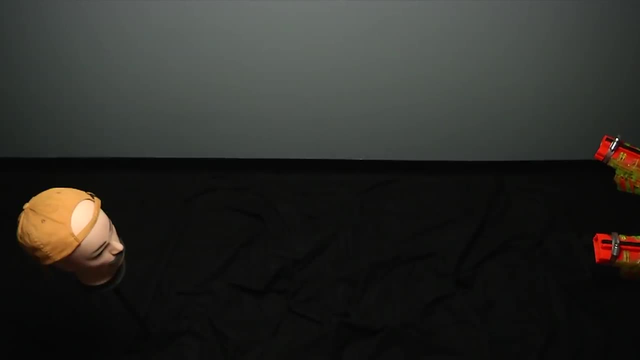 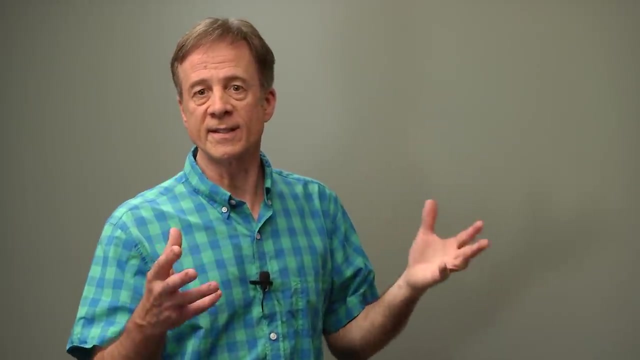 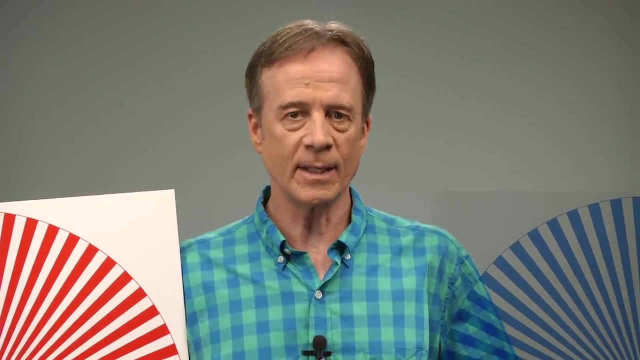 Reflected sound arrives at our ears later than direct sound, even though it started out at the same time, because it's traveling farther And this wall is only one flat surface. There are at least six in the average room And that's a lot of reflected sound. But why is reflected sound bad? I'll demonstrate. 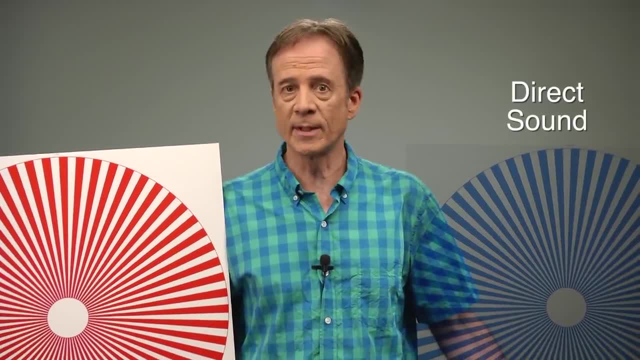 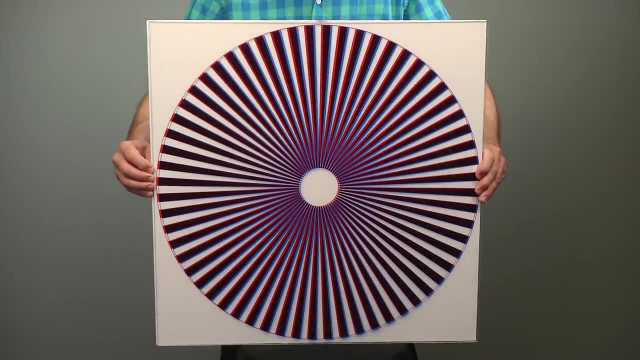 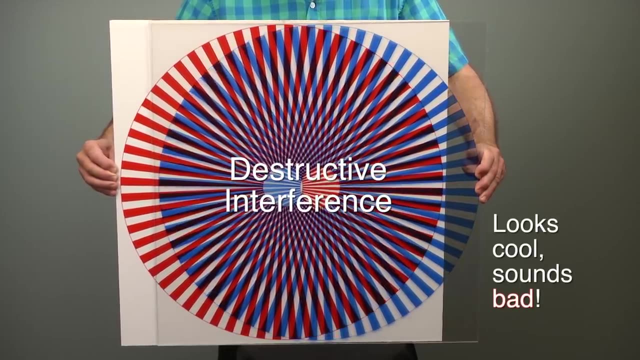 using these two identical patterns. The blue pattern represents direct sound waves and the red pattern represents reflected sound waves. They start out together, But when I move the red one backwards, like a delayed sound reflection, it creates destructive interference patterns, which changes the original sound wave. 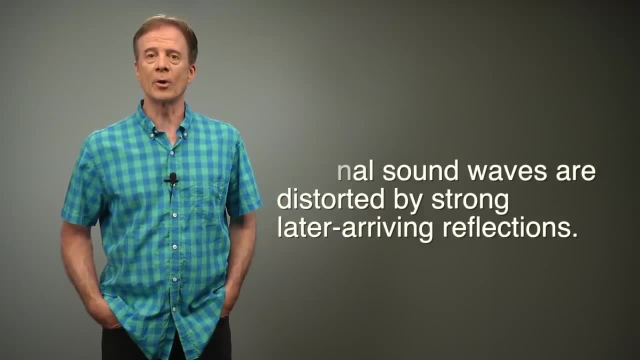 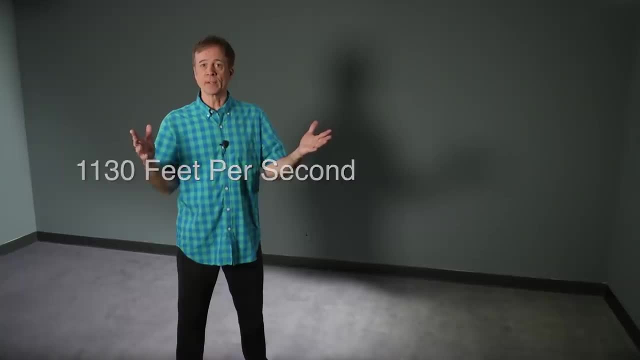 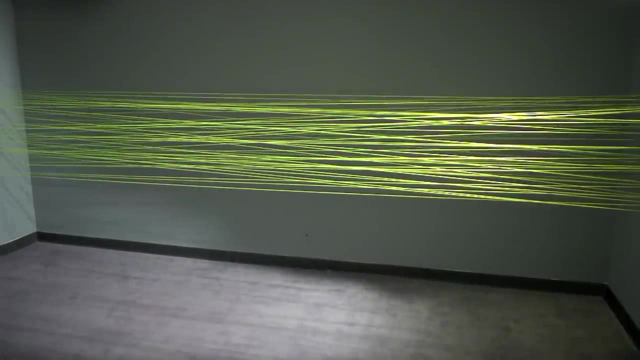 Here's the problem: Original sound waves are distorted by strong later-arriving reflections. Also, sound travels really fast, about 1130 feet per second. A sound wave will bounce back and forth between these two walls about 60 times in one second. 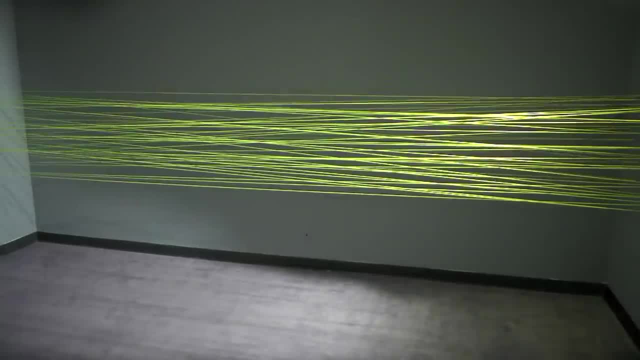 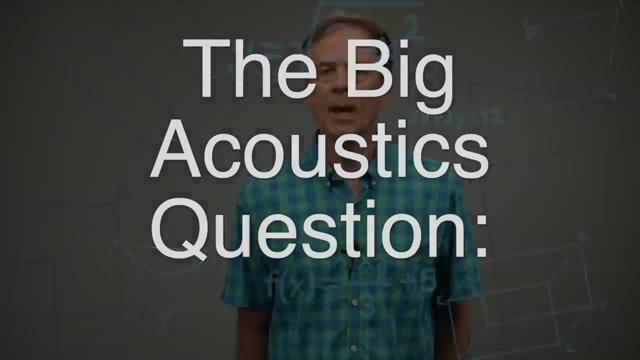 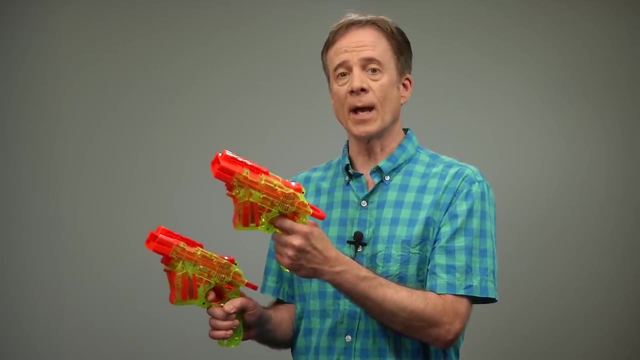 Sound travels so fast it fills a room almost instantly. And this is only one bounce angle. Every room has thousands. How can we make our rooms sound better? Remember our Nerf guns. I'll shoot these at the same time, again representing a sound wave bouncing off a wall. 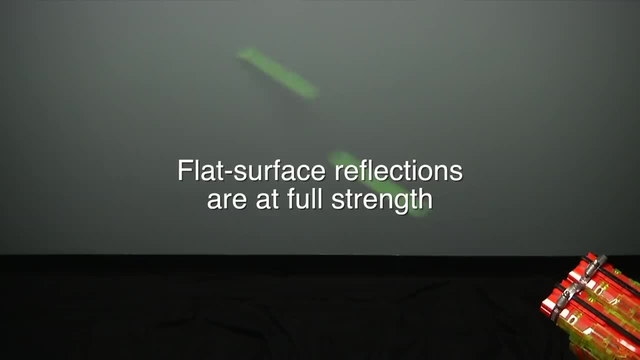 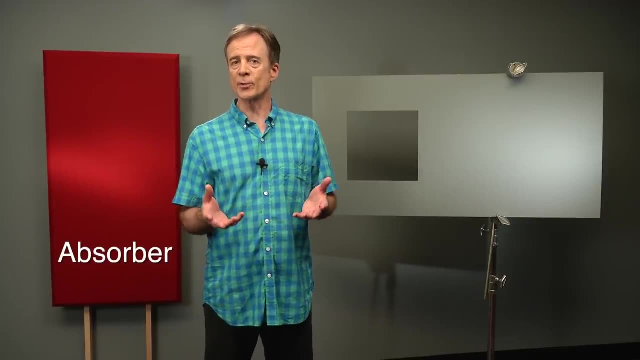 Both discs bounce together in the same direction, which means the reflected sound is at full strength. Now let's use the first of our two acoustical tools, an absorber, to reduce the strength of sound bounces To a sound wave. an absorber looks a little like a hole in the wall, so